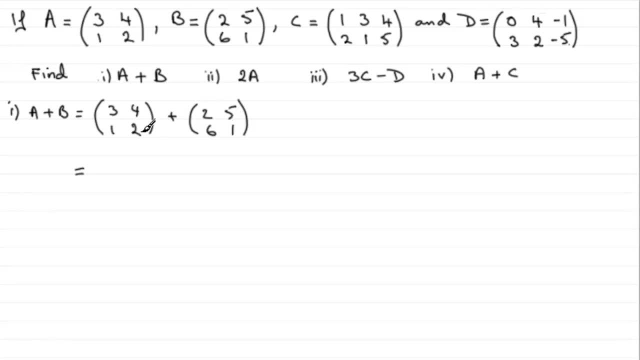 the same dimension. In other words, the dimension of this matrix is a 2 by 2 matrix, as I explained in my first video: Two rows, two columns, And we're adding it again to another two rows by two column matrix. So they've got the same dimensions And the result is a matrix. 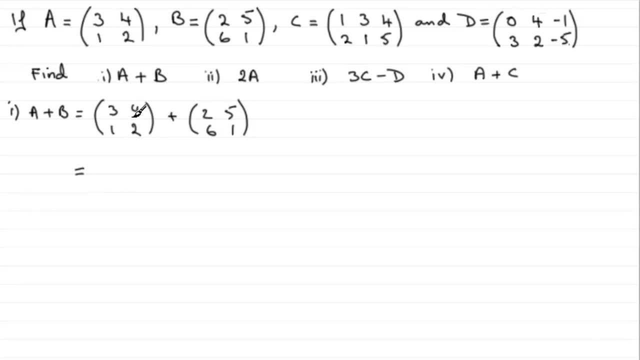 with the same dimensions, a, 2 by 2. And what happens is we just add element with element. So in other words, we've got 3 added to the 2. here gives us 5.. And then 4 plus 5 gives. 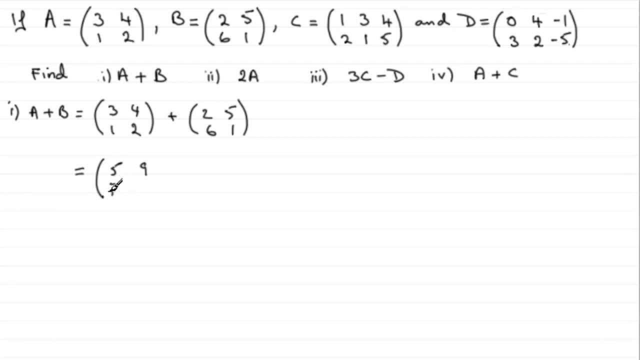 us, the 9. 1 plus 6 is 7. And 2 plus the 1 is 3.. Our 2 by 2 matrix. Now it's pretty obvious why we do this, But I'm just going to step back. 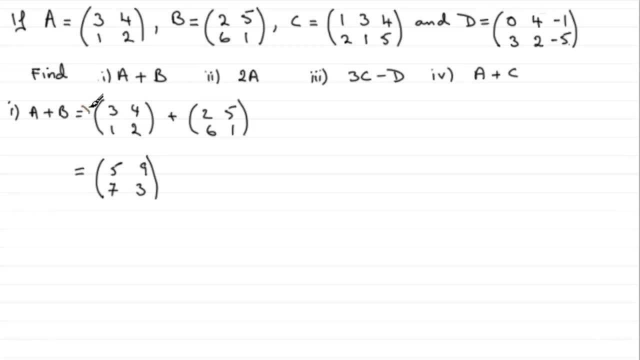 I'm going to give you an example. Suppose we had two countries, say X and Y, And they were given so many golds and so many silvers. We'll have a G for gold and S for silver on a particular day in the Olympics. And then we've got another matrix here giving us the 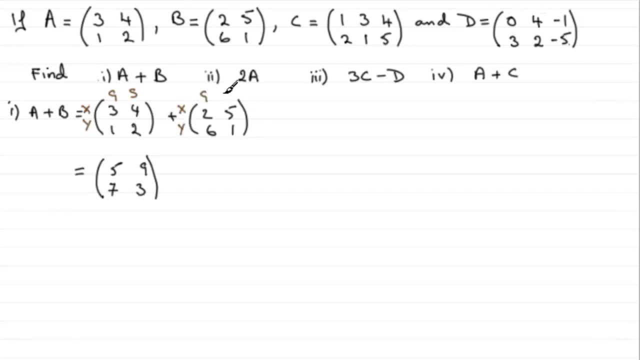 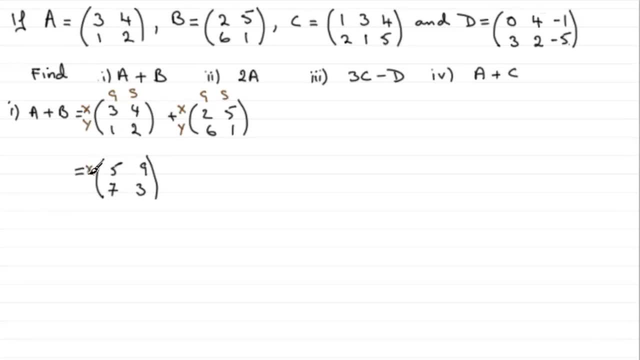 3 and the 2, for instance, it's telling us that country X got 5 golds over these two days And we can fill in the outer values here. So hopefully you can see that this is why we would add two matrices in the way we do. 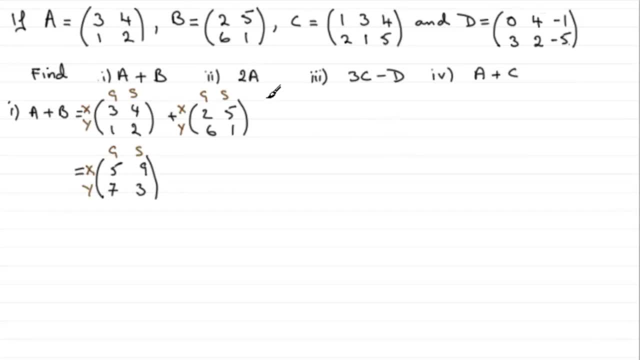 OK, let's just now go and try example 2.. Now in example 2, we've got multiplication by scalar. We've got to do 2 times the matrix A, So we put the 2 there and then we've got. 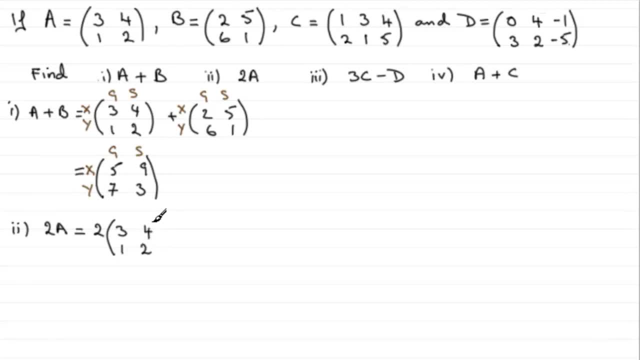 the matrix A, which is 3,, 4,, 1,, 2.. And if you're doubling a matrix, you're basically adding it twice over. So if we were to add this matrix twice over, we would end up with 6,, 8,, 2, 4.. So what we do is just simply multiply the scalar with each of the elements. 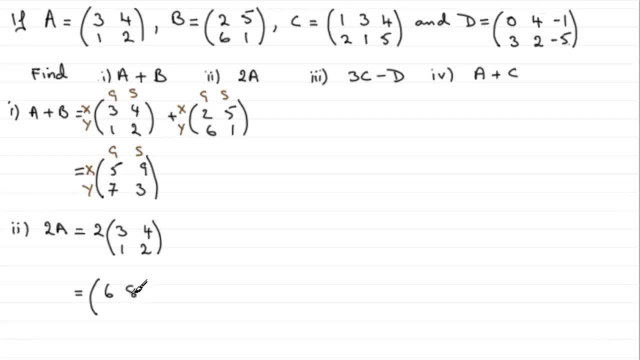 in the matrix. So we get then 6, 8, 2, 4.. 8,, 2, 4 for 2A. Now I've shown you how we can do addition. but subtraction is just exactly the same, Obviously just subtract element with element. So in example 3, I've 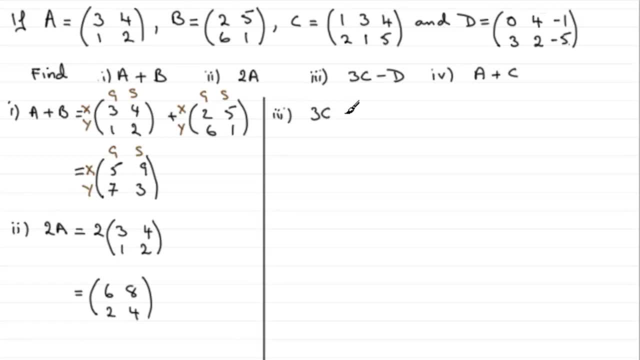 got an example here where we've got to do 3 times the matrix C minus the matrix D. So you might like to pause the video and have a go at this one, just for a bit of practice. OK, let's see how you got on. Well, I'm going to show the working. first of all, I'm going 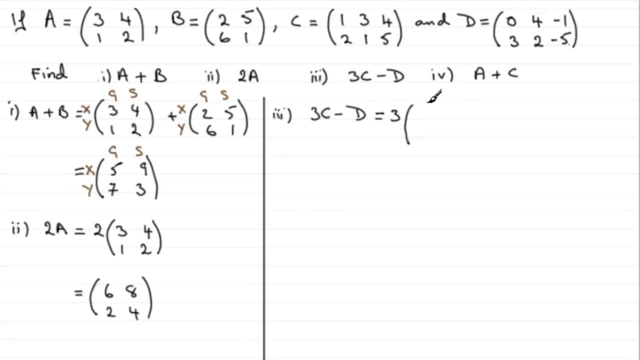 to write down that we've got 3 times the matrix C. Matrix C is 1, 3, 4, and 2, 1, 5.. And then we subtract the matrix D, which is 0, 4, minus 1, 3, 2, minus 5.. So if we work out what 3C? 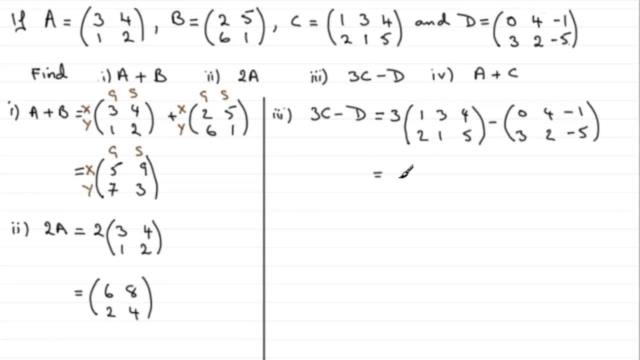 is, first of all, We do 3 times each of these elements And that's going to give us 3,, 9, and 12 on the top row, And then 6,, 3, and 15 on the bottom row, A matrix with dimensions 2 by 3.. And 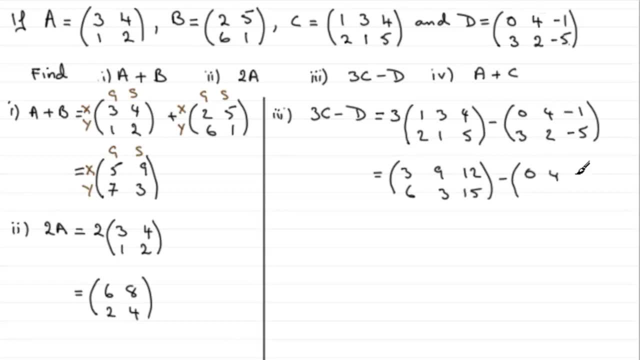 we are subtracting again a 2 by 3 matrix. So it's possible to do this Now. if we subtract each of the elements from one another, We end up with 3. take away 0 is 3.. 9 take away 4 is 5.. 12 minus minus 1 is 13.. And then 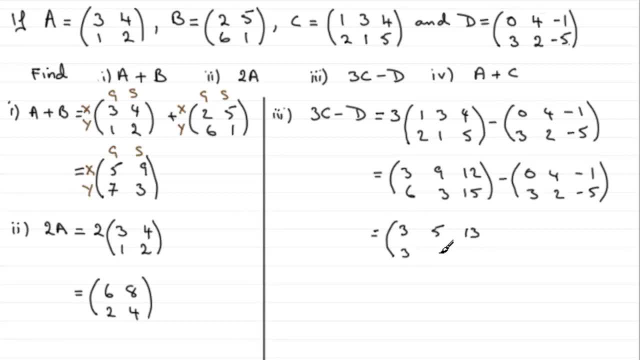 6 minus 3 is 3.. 3 minus 2 is 1. And 15 minus minus 5 is 20.. OK, so 3C minus D. Now for the last one part, 4.. We've got to work out what A plus C is.